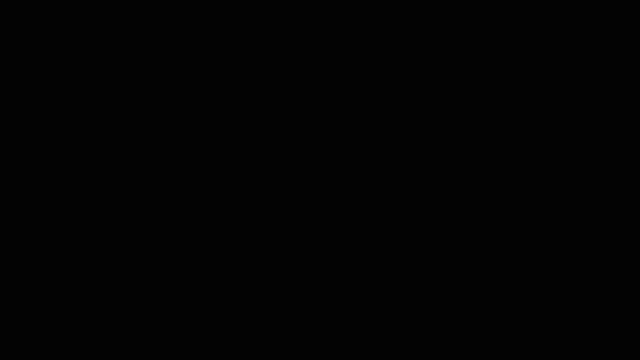 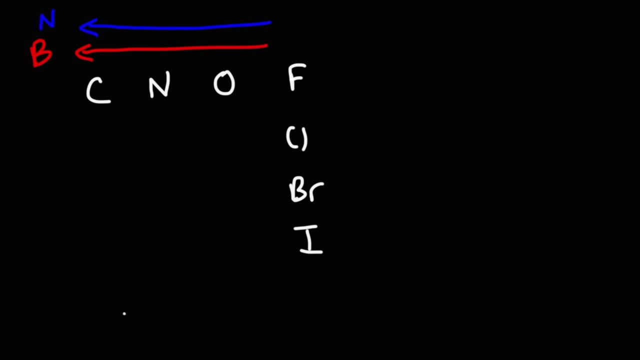 Nucleophilic strength. Nucleophilic strength strength also increases towards carbon. So what this means is that the methyl carbanion is a better nucleophile than the amide ion NH2-. That's a better nucleophile than hydroxide, which is a better nucleophile than fluoride. Now, in a protic environment, base strength doesn't mirror nucleophilic strength, but in an aprotic environment it does So. in an aprotic environment, base strength goes towards fluorine. Nucleophilic strength also increases towards fluorine. 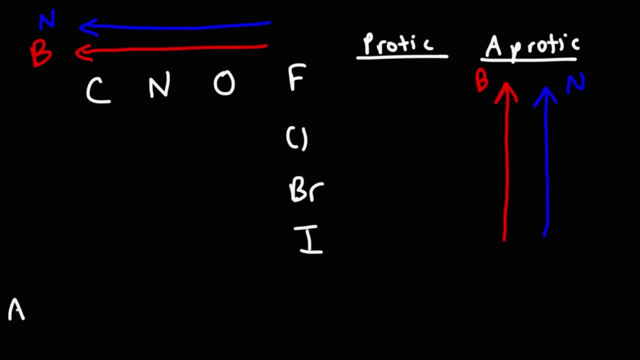 So in an aprotic solvent. what this means is that fluoride is a better nucleophile than chloride, which is better than bromide, and that's better than iodide. Now, in a protic environment, fluoride is still the stronger base, but 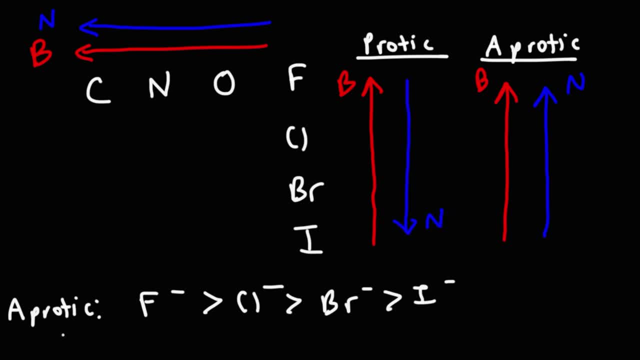 iodide is going to be the better nucleophile. So what this means is: let's say, if the solvent is like water or methanol, or it has hydrogen bond in it, that's going to be a protic solvent. In a situation like that, iodide is going to be the better nucleophile than. 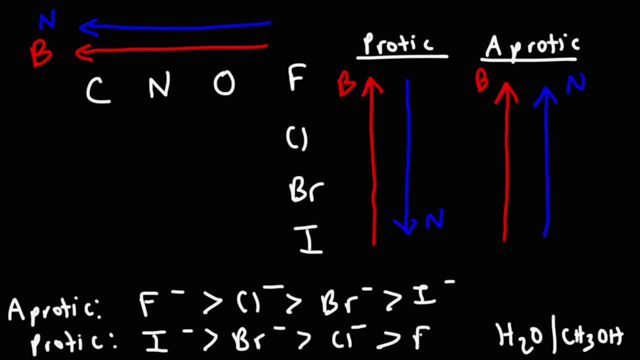 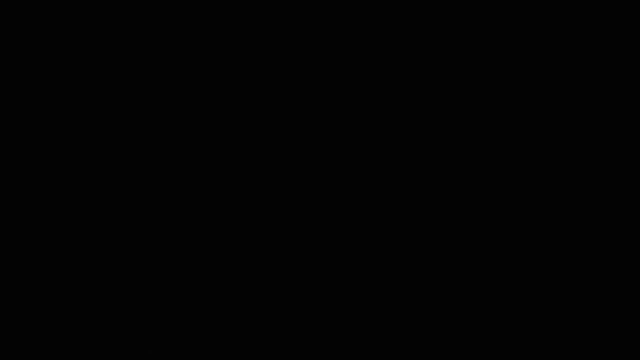 bromide, which will be better than chloride, which will be better than fluoride. So iodide behaves as a better nucleophile in an aprotic environment, but fluoride behaves as a better nucleophile in an aprotic environment, protic environment. so here's a question for you: which one is the better? 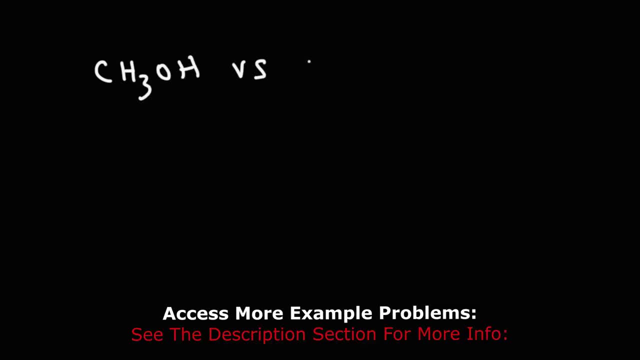 nucleophile, methanol or methoxide. what would you say when comparing similar atoms? nucleophilic strength typically correlates to base strength. methoxide is the better base than methanol and it's also going to be the stronger nucleophile, so it's going to be methoxide if you're comparing an oxygen that is neutral. 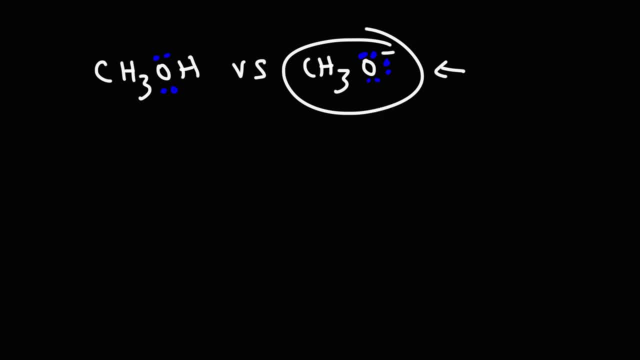 versus an oxygen with a negative charge. the one with a negative charge will typically be the stronger nucleophile. now what if we were to compare hydroxide with the acetate ion? which one is a better nucleophile? so in both cases we're dealing with an oxygen. 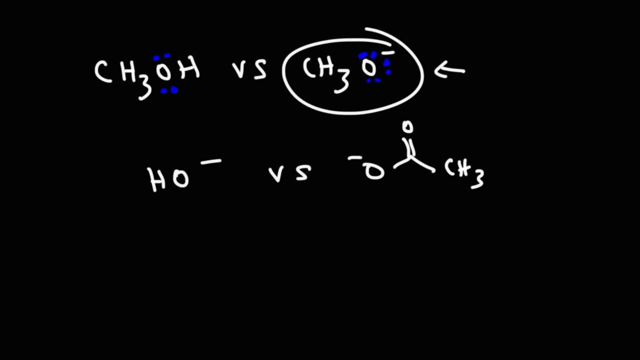 with a negative charge. in this case, nucleophilic strength will mirror base strength. if we look at the conjugate acid of hydroxide, which is water, it has a pKa of 15.7. acetic acid has the pKa of around 4.75. 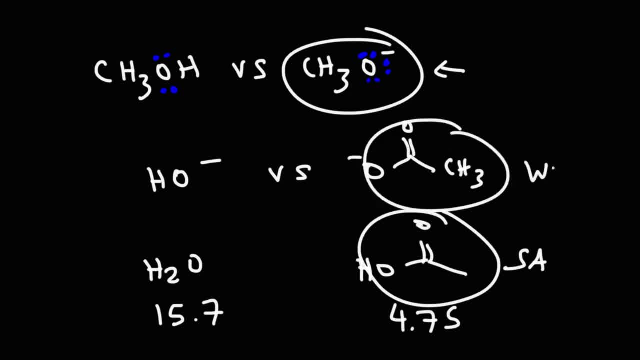 so this is the stronger acid, which means this is the weaker base. therefore, hydroxide is the stronger base, which means it's going to be the better nucleophile. so the answer is hydroxide: it's the stronger base and also the stronger nucleophile. now what about comparing? 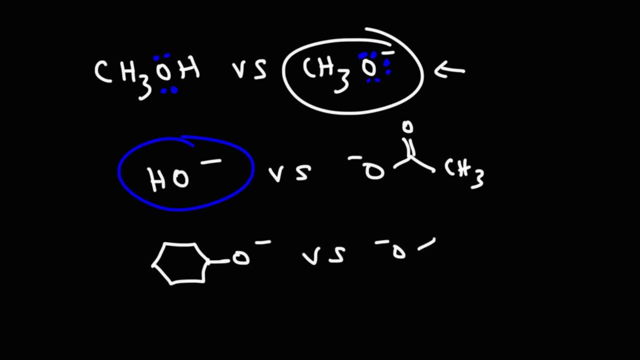 phenolphthalein and acetic acid. if we compare hydroxide with acetic acid, which one is the stronger nucleophile? the pKa of Phenol is ten, 4c acid, its 4.75. the pKa of phenol is ten for acidic acid. it's for four, point cinema. 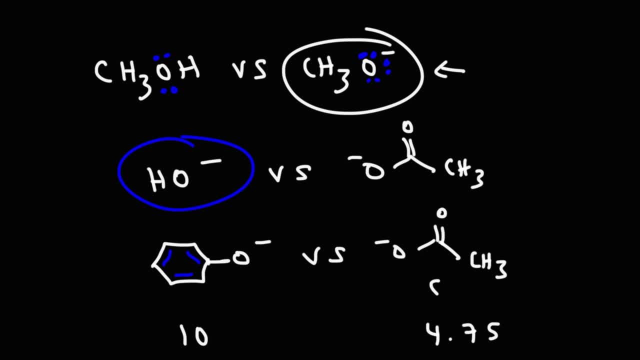 so this is going to have the stronger conjugate acid, which makes it a weaker base. this has the weaker conjugate acid, which makes it the stronger base, and it's also going to be the stronger conjugate initializer, stronger nucleophile. so in most cases, base strength typically mirrors. 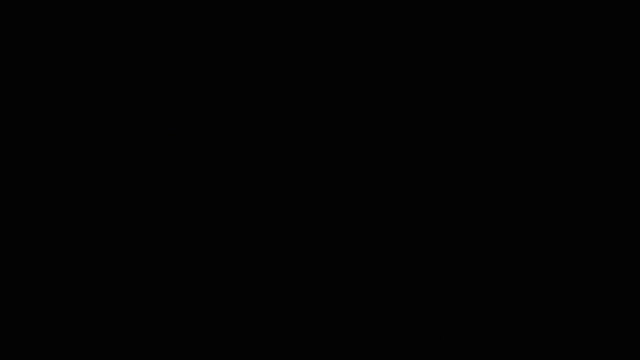 nucleophilic strength. now what about comparing ammonia and water? which one is going to be the stronger nucleophile? so we're comparing different elements in the same row. if you recall, nucleophilic strength increases towards the left, so it's going to be ammonia. now what if we compare the thiolate ion with an alkoxide ion? 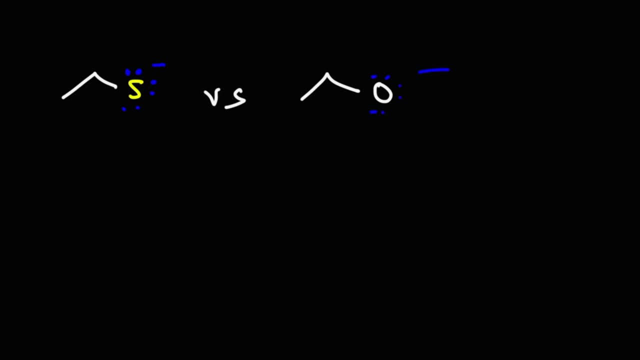 which one is the better nucleophile. so we're comparing oxygen and sulfur. we need to define the solvent when you're dealing with atoms of different size. so let's say in water which one is going to be the better nucleophile in water. water is a protic solvent in a protic solvent. 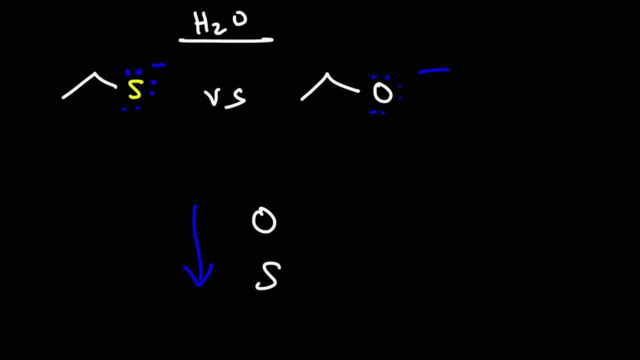 nucleophilic strength increases towards iodide increases as you go down. so sulfur with a negative charge it's going to be more nucleophilic than oxygen with a negative charge. now, let's say, if we have a similar situation but in an a protic environment, 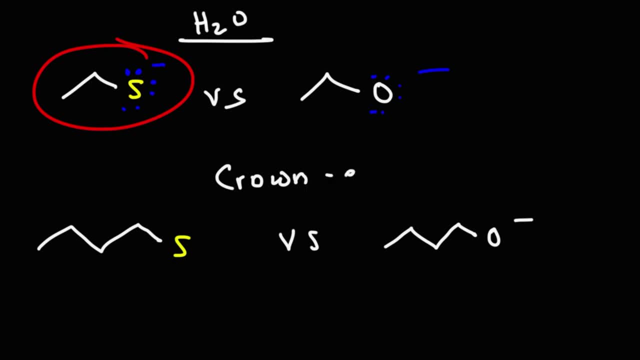 let's say if this was dissolved in a crown ether. a crown ether is an, a protic solvent. in that case, which one would you say is the better nuclear file? in an, a protic environment, oxygen with a negative charge will be more nucleophilic than a. 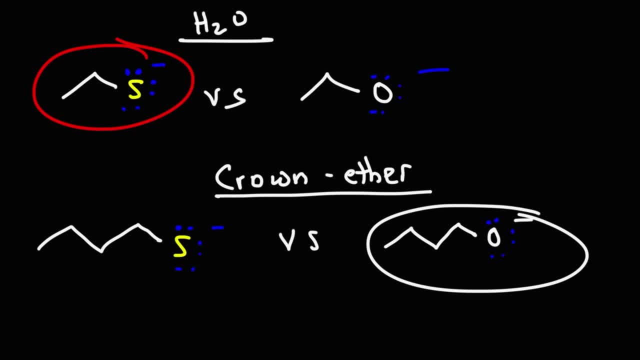 sulfur atom with a negative charge. so that's basically it for this video. hopefully I gave you a good idea in terms of how to identify which compound is going to be more nucleophilic. so just to review, if you have a neutral molecule with one that has a negative charge, typically the one that has the negative 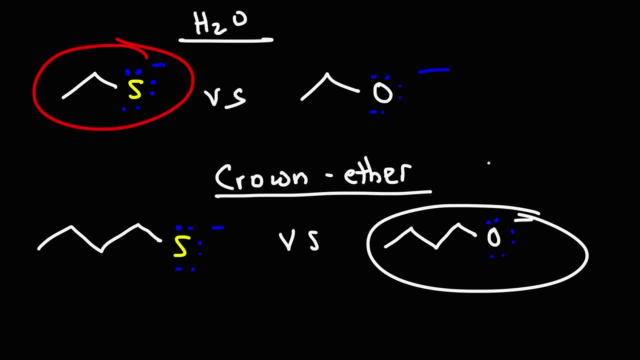 charge is going to be more nucleophilic and nucleophilic strength increases towards the left. it also increases downward in a protic environment, but it increases upward in an aprotic environment. now for those of you who are interested in getting more practice examples on SN1, SN2, E1, E2 reactions, I do 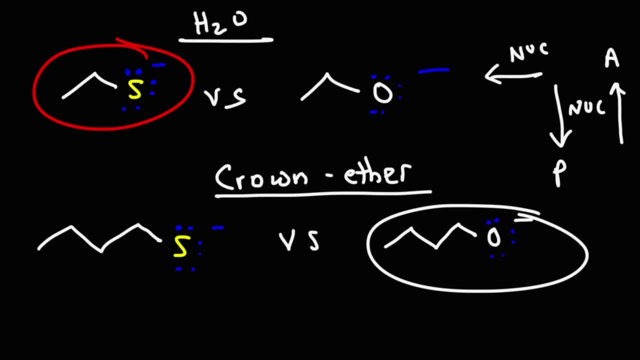 have a practice test available and I'm gonna post it in the description section below, so feel free to check the links below this video for those of you who want more additional resources in preparation for your next organic chemistry exam.